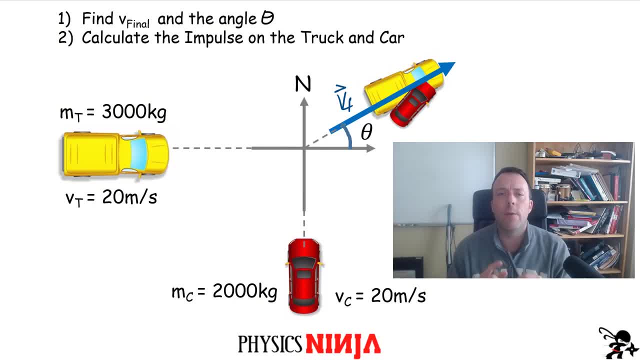 Now, hi everybody, Physics Ninja here. Today what I want to do is look at a perfectly inelastic two-dimensional collision. All right, what we have here is a truck traveling eastbound and a car traveling northbound. They are going to collide with one another and lock up. So after the 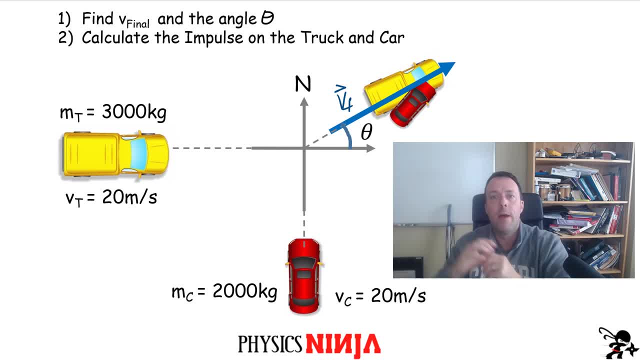 collision they all move together as one big chunk of stuff And that means that both objects, after the collision, travel at the same velocity And in this case it's going to be at some angle relative to the x or the east direction. I have a couple questions associated with this problem. First, 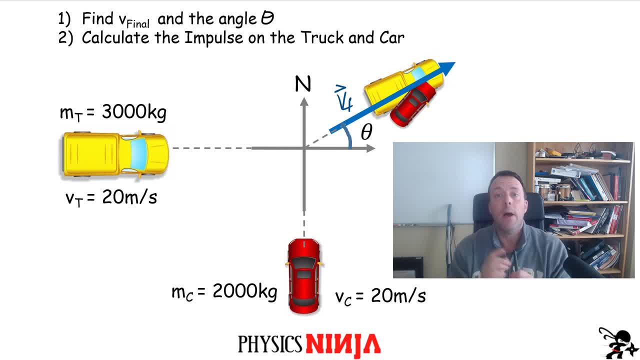 how do we find this final velocity as a vector? Okay, what's the magnitude and what is the direction that the chunk slides off after the collision? In addition to that, we're also going to look at the impulse on the truck and the impulse on the car, Again as a two-dimensional. 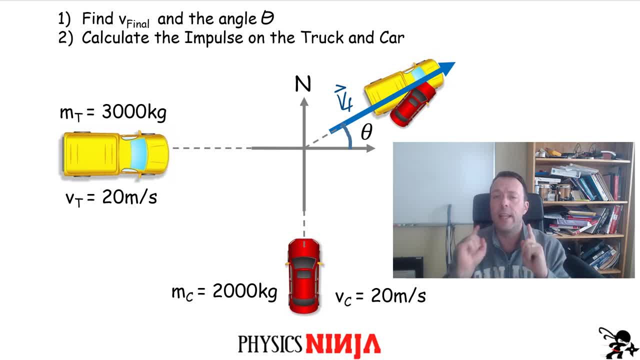 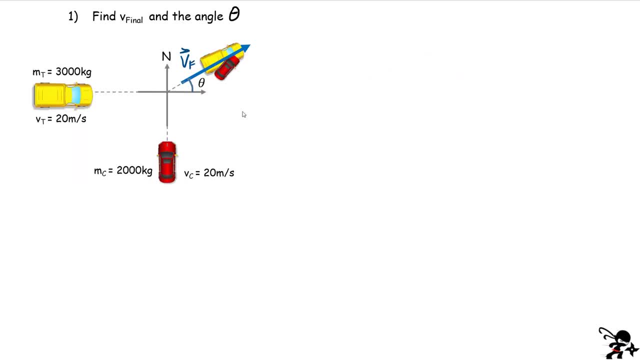 problem. All right, the best way to support Physics Ninja is to like this video and to subscribe to my channel. All right, let's get started. All right, so our truck has a mass of three kilograms, traveling at a speed of 20 meters per. 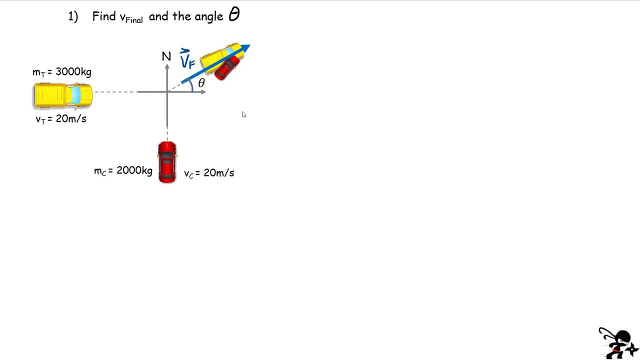 second, traveling east, And the car has a mass of 2,000 kilograms traveling north at also 20 meters per second. All right, first questions: how do we find v final and this angle theta if, after the collision, we have our both objects locked together, moving together as one? 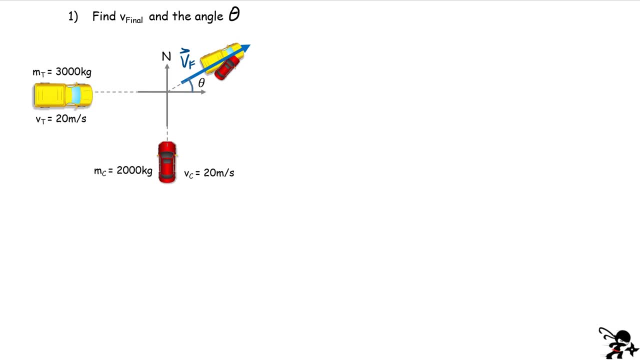 All right. so the key concepts for this one is: we have a conservation of momentum. Okay, so let's just write that down. And why do we have conservation of momentum for this collision? there is a force acting on the truck. there's also a force acting on the car during the collision. 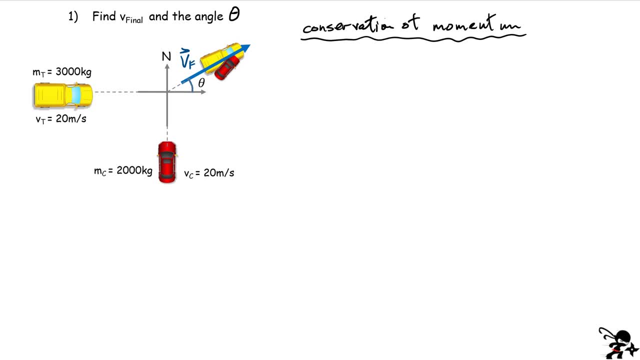 But that's it right. These are action reaction pairs and there's no external force acting on the system, So which means that the total momentum of the system which is composed of the car and the truck before the collision has to be equal to the same momentum of the car before the collision. 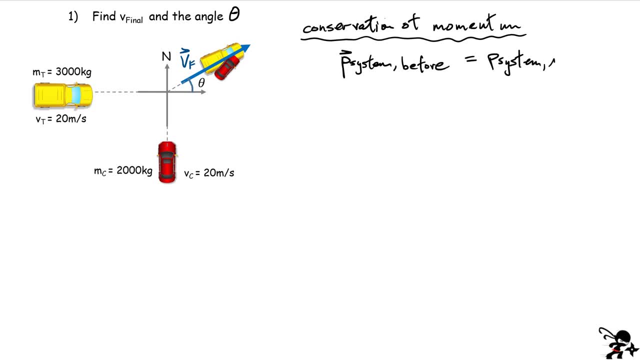 And again the same thing after right, if I look at the total momentum of the system, after both those values must be the same. And again, my system here is made up of the truck and the car. So let's do that Now. since this is a two dimensional problem, you have to break things down into components. 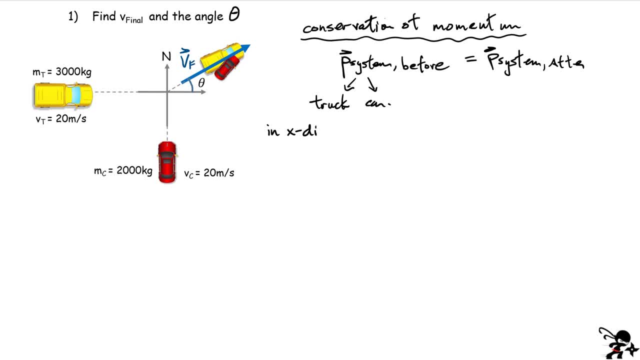 So what I'm going to do here is I'm going to look at the x direction separately from what I do in the y direction. All right, so in the x direction I'm going to write conservation of momentum, And in the y direction 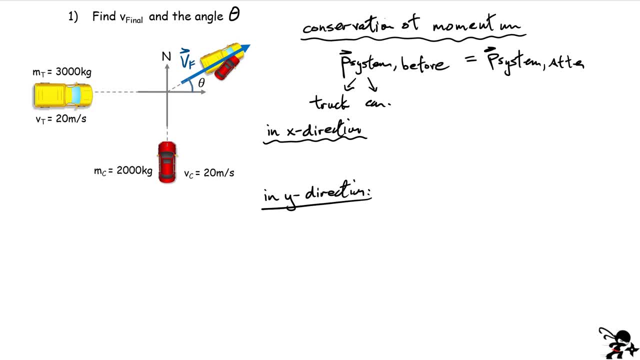 I'm also going to write an expression for conservation of momentum. So what do we have in the x direction? the only thing moving in the x direction before the collision is the truck. So what I do is I write the total momentum of the truck, So it's the mass of the truck multiplied by this velocity, Vt, which is 20.. Okay, 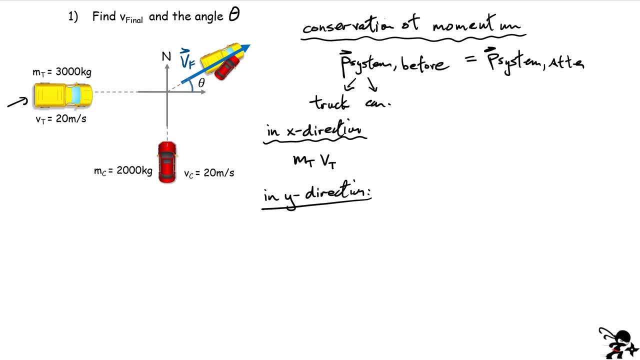 And since this is moving here to the right, I'm going to take that to be a positive value. Okay, so I simply write it like this: This must be equal to the total momentum of the truck. This is the total momentum of the system after the collision. 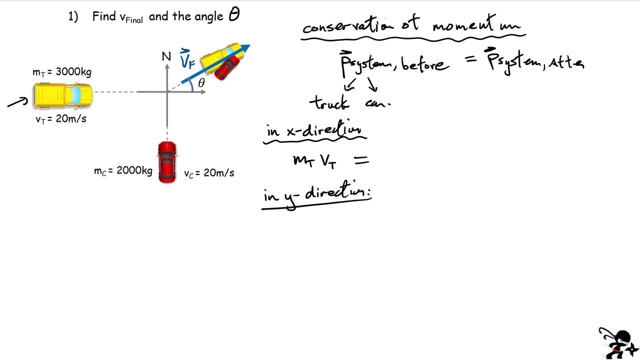 So what do we have? We have a velocity here that's going off at an angle. I can break that velocity down into two components. This is my velocity in the x direction, after which I can write as Vf cosine of the angle theta. 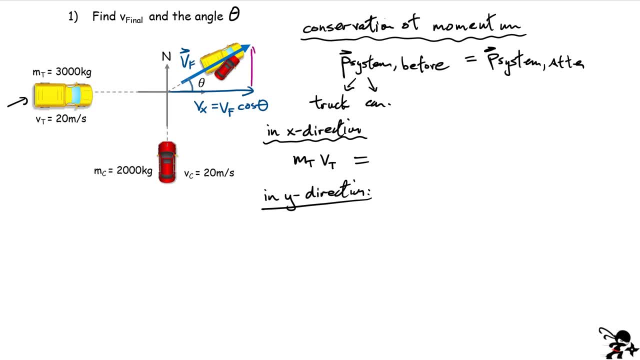 And I also have a component of the velocity here that is in the vertical direction here or in the north direction. This is what I would call Vy, So I'm just using some trigonometry. I can write it as Vf: the length of this one multiplied by sine of the angle theta. 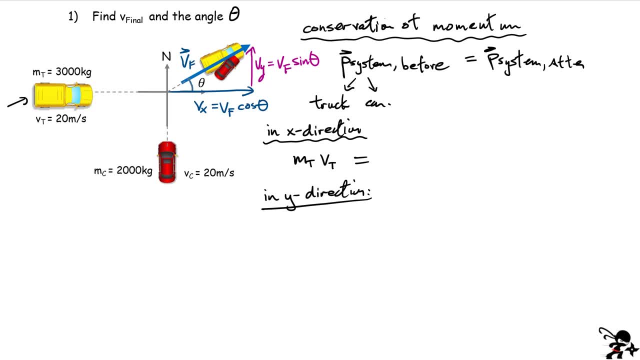 All right, I'm off to a pretty good start, So let's go back to my expression now in the x direction. So what is the momentum in the x direction? Well, remember, everything here is locked together and it's moving together. 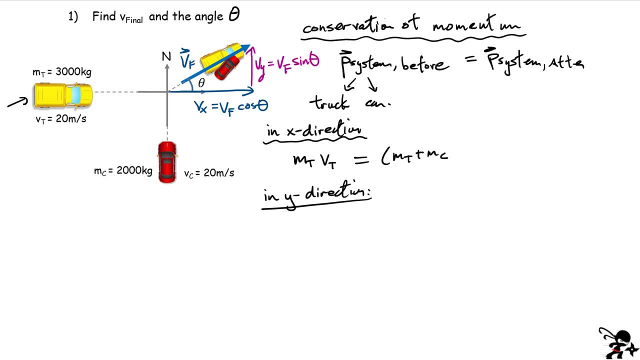 So it's the total mass, so mass of the truck plus the mass of the car, And it's moving in the x direction with this velocity. So I would write this as Vf cosine of the angle theta. Here is equation one. Let's now look at the conservation of momentum in the north direction, in the vertical direction. here. 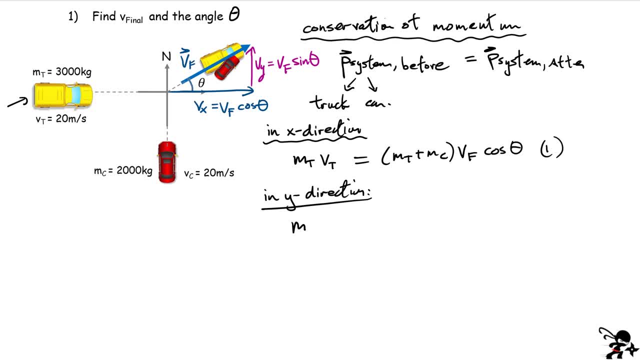 So what do we have? Well, I have a car that is moving up, and it's moving at some velocity- Vc- which is 20 meters per second. The truck doesn't have any momentum in this north direction, So that's it. 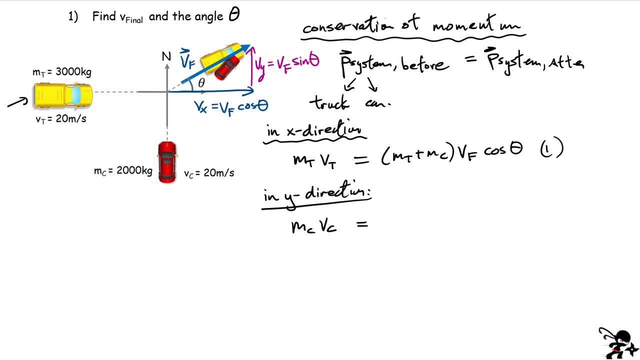 Before the collision. that's all I have. After the collision I have this big chunk of stuff which has a mass of The truck plus the car And it has a component of velocity that is moving north And that component is Vf sine of the angle theta. 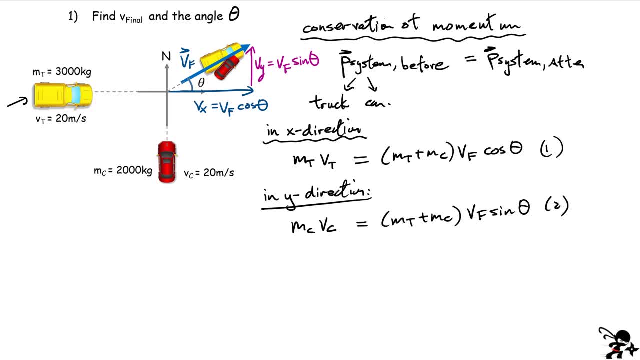 Okay, so we have two equations. Guess what? We have two unknowns. Can you guess what the unknowns are in this problem? Okay, the unknowns are Vf. what is the magnitude of this velocity? and also the angle, theta. 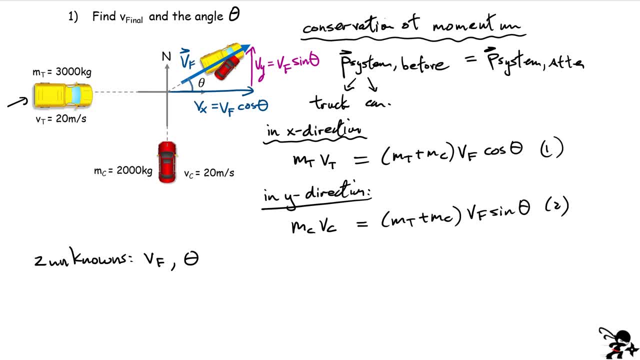 So what you have to do now is you have to do a little bit of algebra in order to solve for this. What you can do is either isolate and substitute Again- we know all the masses, We know this Vt and Vc. 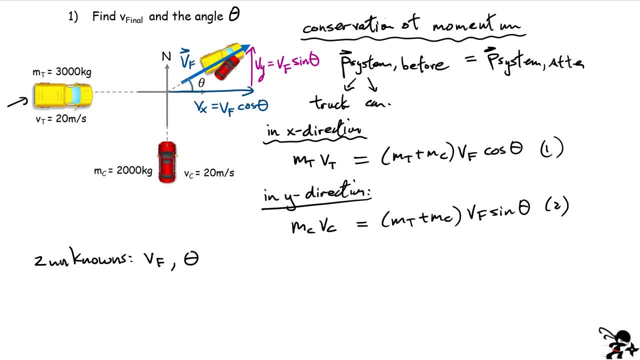 Those are 20 each. The easiest way for me to solve that is, if I do, equation 2 divided by equation 1.. If I do that, look what's going to happen: The Vf's are going to cancel and I'm going to get simply one expression in terms of theta. 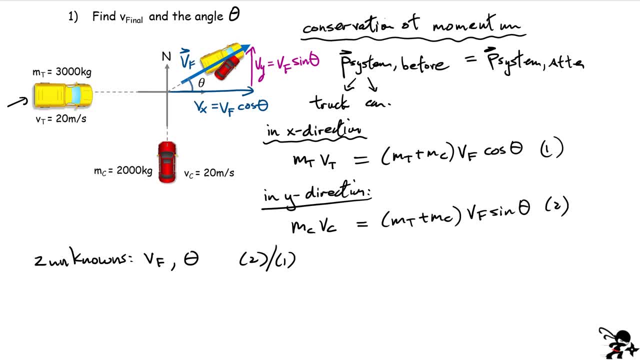 So let's go ahead and do that. So on this, again I'm doing equation 2 divided by equation 1.. So we get mc Vc Divided by mt Vt. Again, we'll make some simplifications in just a minute. 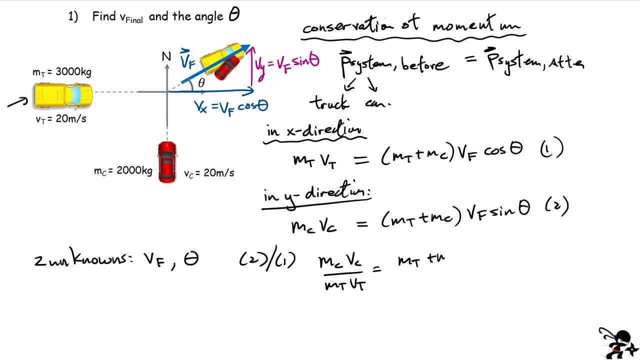 Let me just write out the entire equations: mt plus mc, Vf, sine of the angle theta Divided by again equation 1, which is up here. Alright, just write this out: Vf, cosine of the angle theta. 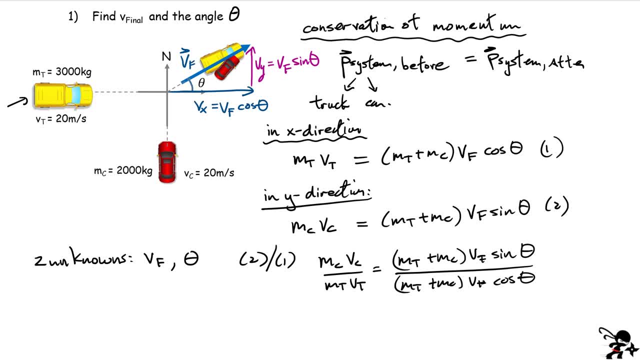 Alright, let's simplify some of the terms here that are the same. First of all, these m total masses are the same for both. Those can cancel out What else. Vf's are the same, And what I'm left here is a sine divided by a cosine. 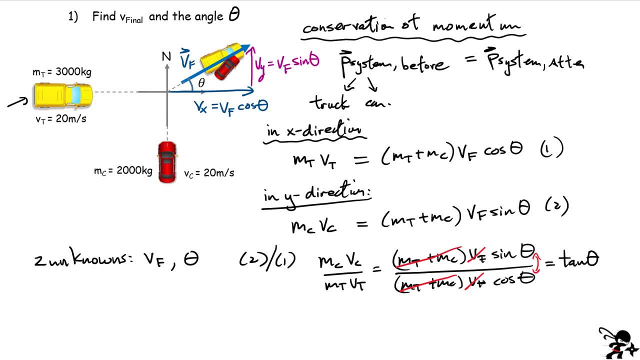 So this right hand side simplifies to tangent of the angle, theta And everything here I can substitute the values. Now, since these have the same magnitude and principle, these also cancel out Right, because both of these guys here are going to be 20 once I substitute the values in. 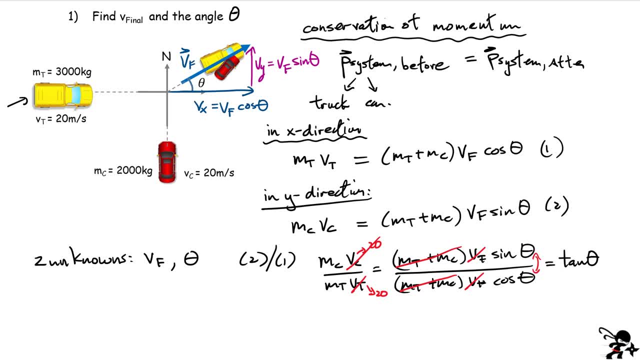 So you could just cancel those out for now. If the speeds were different before the collision, then I'd still have both of those terms. So we're left here with one final expression. Now we have tangent of the angle. theta right here is equal to the ratio of these masses. 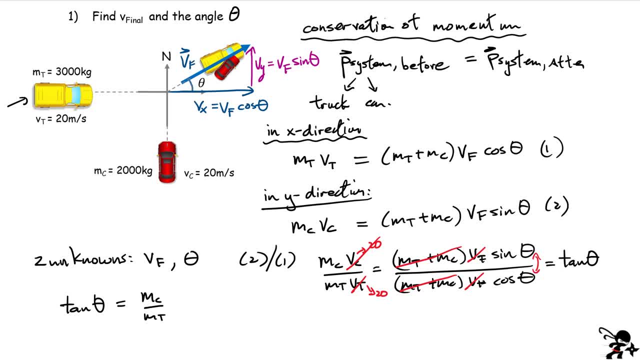 In this case, because those initial speeds were the same. Now we substitute the values: Mass of the car is 2,000.. Mass of the truck is 3,000.. Cancel a bunch of those out. Cancel all the zeros. We're left with 2 over 3.. 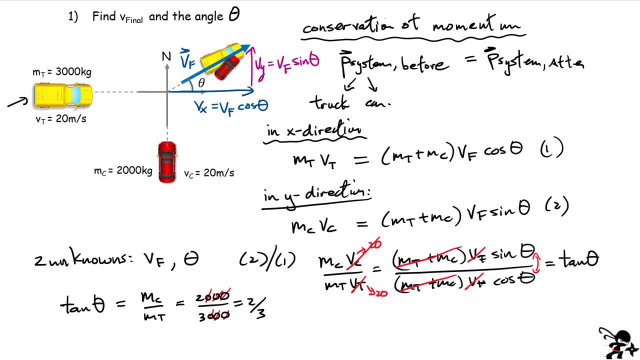 So all we have to do now is take an inverse tan. All right, so we get that. the angle theta- you do that in the calculator should get something that is like 33.7.. Let's just keep three significant figures for that one. 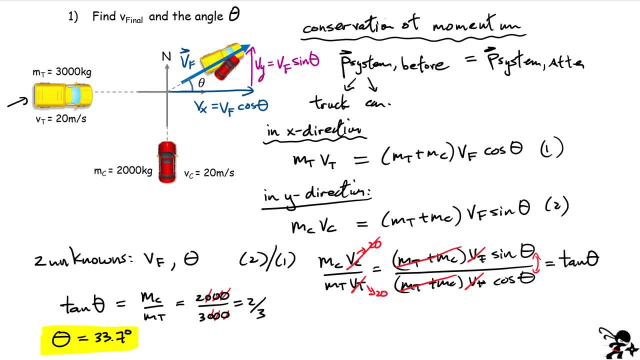 All right. so that's how you find the angle theta. Now how do you go back and solve for, for example, the speed VF? What you can do now is use any of the equations. I can either use equation 1 or equation 2.. 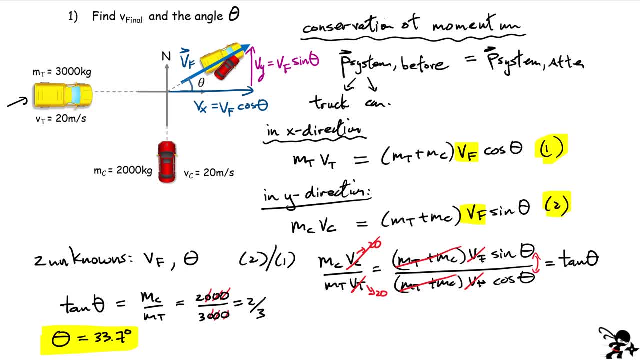 It doesn't matter, And you simply substitute the angle theta for 33.7.. So let's just use equation 2 right here And let's isolate for VF. So my expression for VF is equal to mass of the car, velocity of the car, divided by the total mass and multiplied by sine of the angle theta. 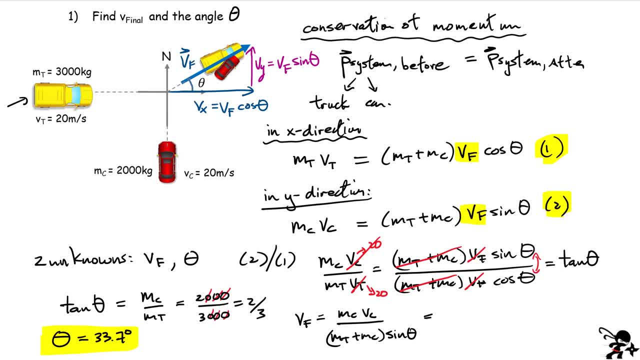 All right, we substitute our values. Mass of the car was 2,000.. Speed of the car: 20. And again the total mass. The total mass now is again 2,000 plus 3,000, because everything is moving together as one. 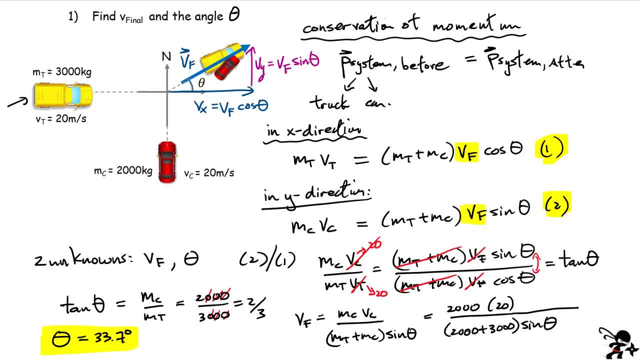 And now I can't forget this important term. This is sine of the angle theta. Okay, at the end of the day you put that in the calculator. Assuming I did everything correctly here, I think I get like 14.4 meters per second. 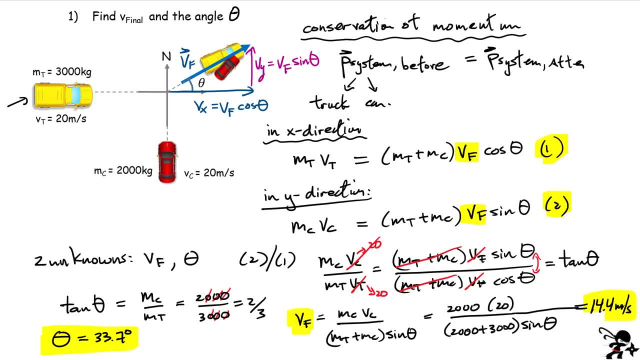 So let's go ahead and highlight that That is our final speed. Okay, so not too bad a problem. Let's go in the second problem now and calculate the impulse on the car. All right, second problem: we now want to look at the impulse on the truck and the car. 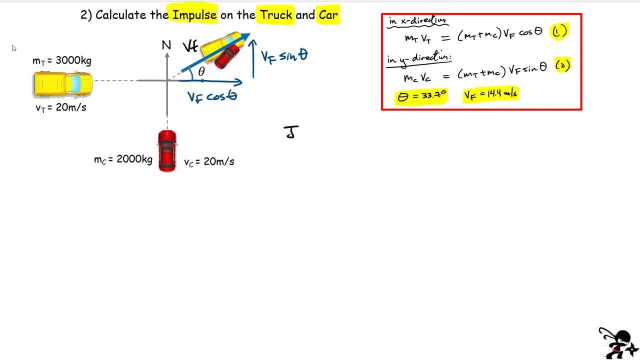 So let's start with one object. Regardless of the object, the impulse you can calculate as the force multiplied by how much time that force is acting on the object, Or you can calculate it using the change of momentum of an object. So for this problem it's probably best to use the change of momentum definition. 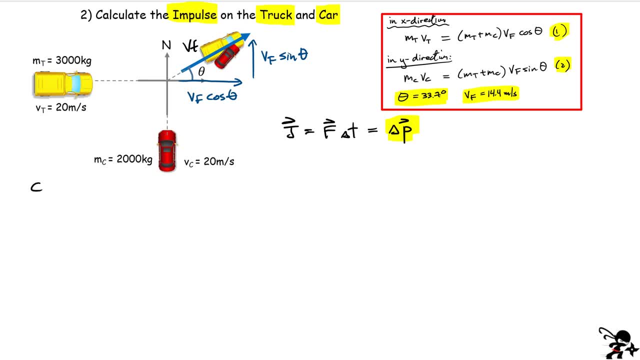 We're going to start with the car, All right. So that means to calculate the impulse on the car. I have to look at the change of momentum on the car. So this is going to be p final of the car minus p initial of the car. 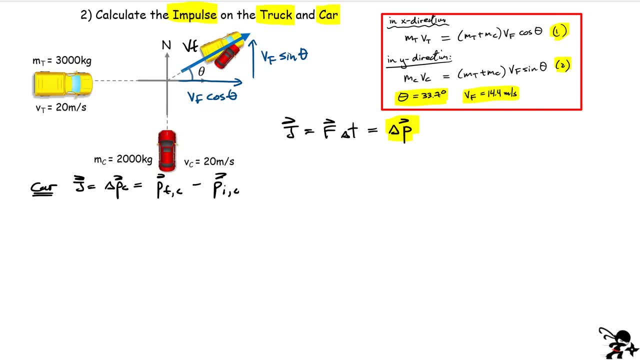 Now, keep in mind, these are two-dimensional vectors, both of these. So how do you write the final momentum of only the car? Well, you'd write it as the mass of the car times its final velocity. The final velocity is vf. 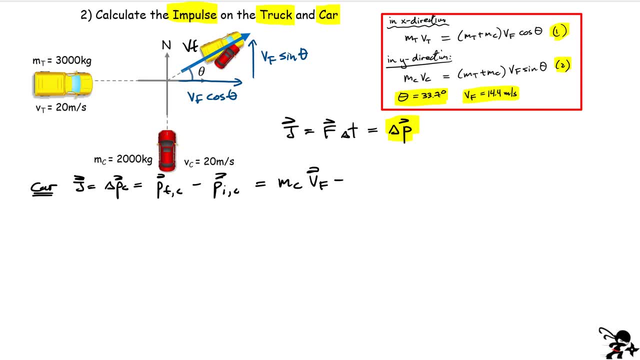 Minus What is the initial momentum of the car? The car is simply moving like this. So it's going to be the mass of the car multiplied by vc, And I'm going to write vc here as a vector. I have to represent it as a two-dimensional vector. 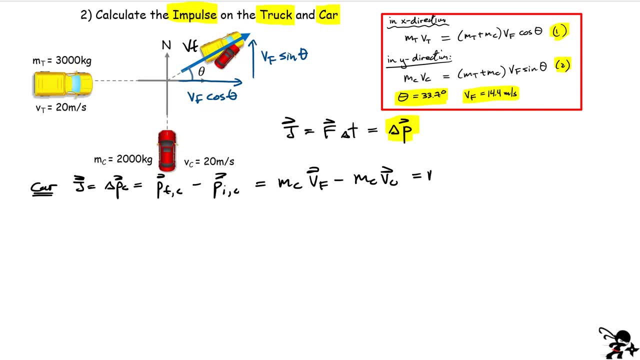 Now let's take this equation one step further. I can factor out the mass of the car. If I do that, let's open up a square bracket And then I'm left with the difference between both of these vectors, V, final of the car, and this second term. here is the initial velocity of the car. 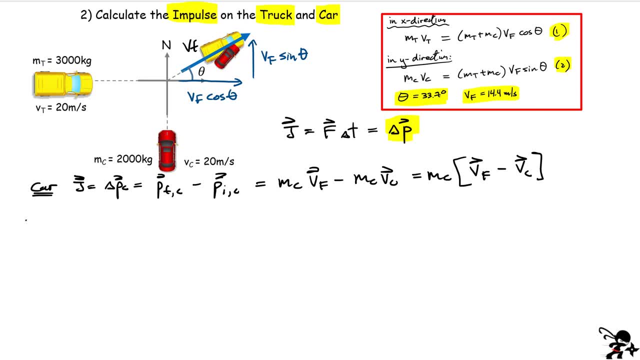 Let's write those as vc. Let's write those as two-dimensional vectors. So the impulse for again the car is equal to mass of the car. All right, How do you write v final? now? Let's open that up. Let's write v final as a two-dimensional vector. 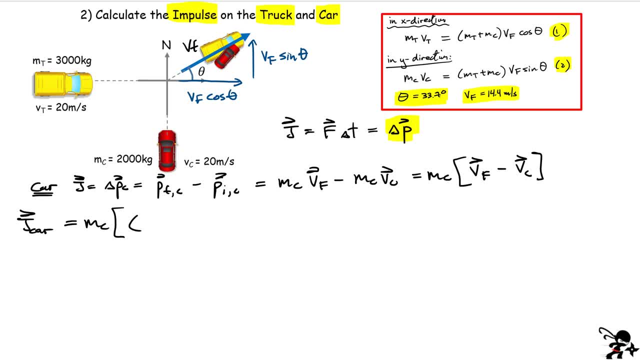 Here is v final. It has an x component and a y component, So I would write it as vf cosine of the angle theta And I'd write vy as vf sine of the angle theta. Good job, Minus. What is the initial velocity of the car? 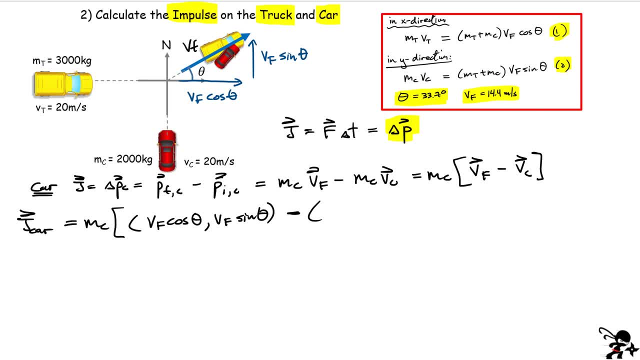 Well, the initial velocity of the car is only in the y direction. It has no x direction. So I have to write zero for the x component And the y component is simply this: vc. All right, This, 20 meters per second. 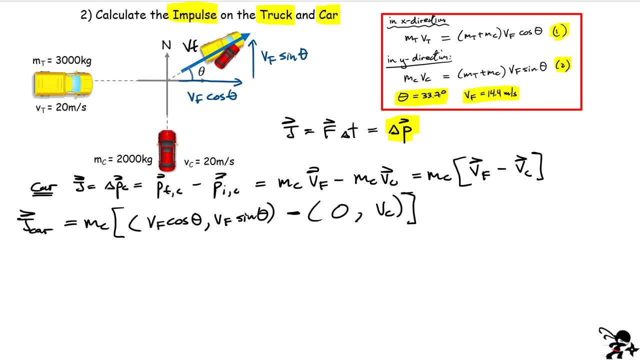 Now you could substitute all the numbers here. All right, I know what the angle theta is. I know what vf is. I'm going to try to avoid that right now because I don't want to get any rounding error. Okay, So let me make sure I don't have any rounding error. 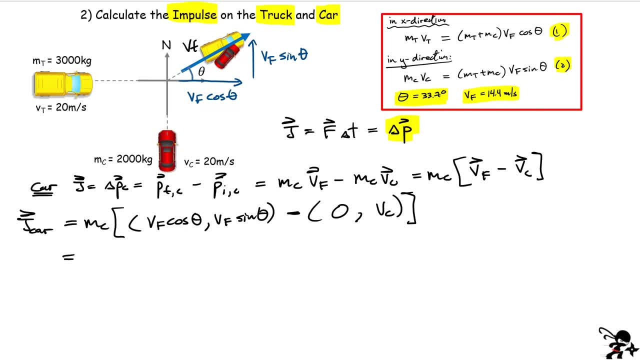 So how do I do that? So how do I take this expression a little bit further? Well, one thing I could do is look at these expressions here: vf and vf sine theta and cos theta- They're actually the expressions that are written right here in the conservation of momentum statement. 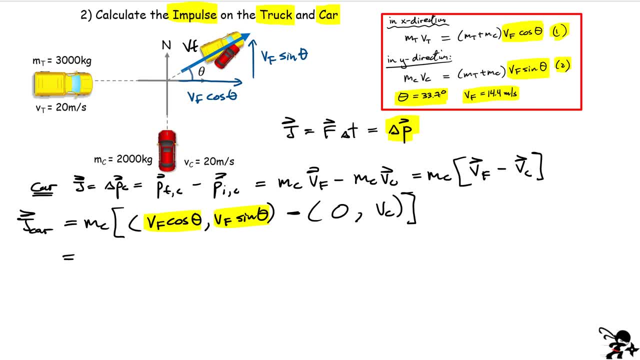 So what I'm going to do. notice, I can write vf, cos, theta, as if I bring this term here on the other side. Let me go ahead and do that, And then at the end I'll substitute the values of the masses. All right? 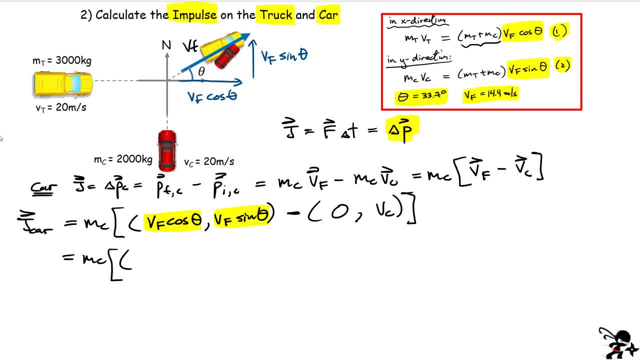 So let me open this up. So instead of vf, cos theta, I'm going to write it as mass of the truck, v of the truck divided by the total mass of the system, mass of the truck plus mass of the car. Now this second term here: instead of vf sine theta, I'm going to write it as mass of the car, velocity, the speed of the car, divided by mass of the truck plus mass of the car. 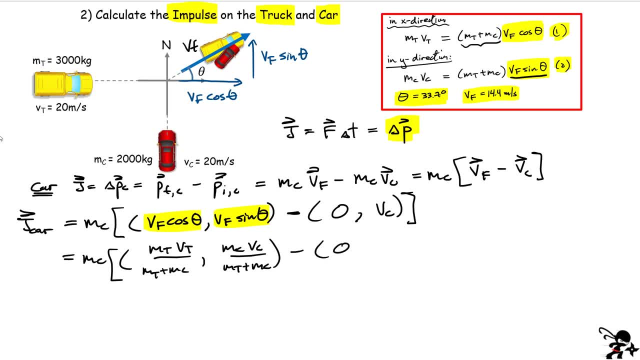 All right, So that is the first vector. The second vector, I'm not going to do anything, All right. So this way I don't have any rounding error, because I truncated this to three significant figures. There may be more, and I just don't want to have any errors whatsoever because I'm trying to show you something that's going to come out of this calculation. 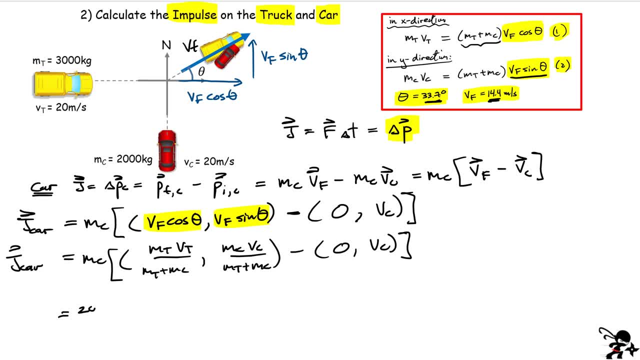 All right, Now we're going to substitute our values. Mass of the car: 2,000.. What else? Mass of the truck: 3,000.. Vt: that's the speed of the truck. That was 20.. 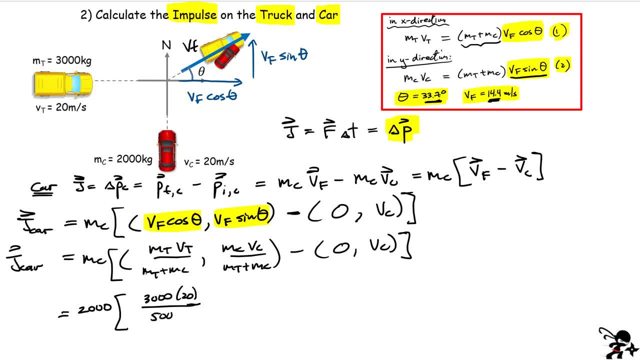 Total mass down here is 3,000 plus 2,000.. I could just write that as 5,000.. All right, Again, now we keep going. This is 2,000 multiplied by 20, over 5,000.. 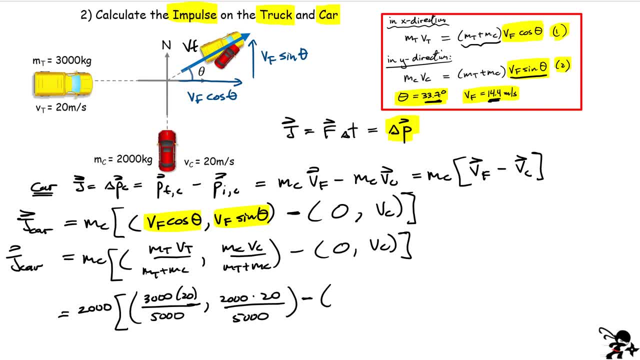 Okay, So that's this first vector Minus zero. And what's that speed? This was 20.. Okay, Now we have to take out our red pen here and just simplify some of these expressions. I can cancel out some zeros. 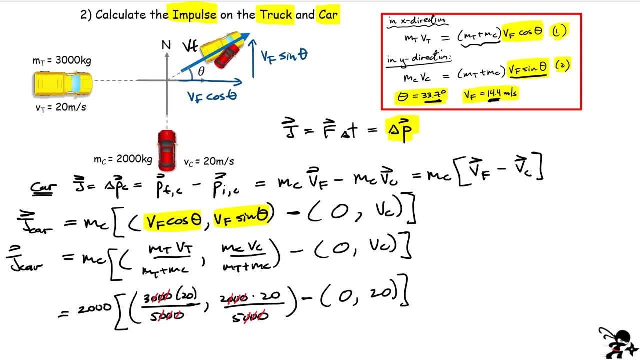 Let's cancel out some zeros: One, two, three. Okay, Now we're going to finish off the problem, So I'll keep the mass of the car outside of the parentheses right here, And let's simplify this. I have 3 times 20.. 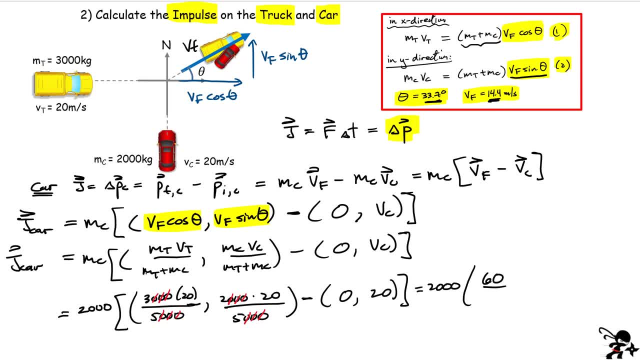 3 times 20 gives me 60 over 5.. Okay, What else? The next term here is 2 times 20.. That is 40 over 5.. And then minus zero. Minus zero and 20.. Okay, 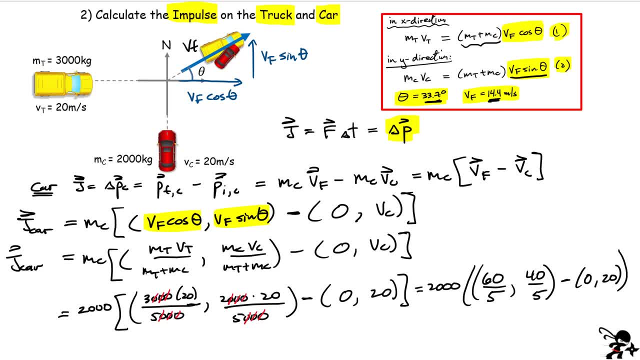 And our last calculation. now We take the difference now between both of those terms, So we have that the impulse on the car is equal to. I'll keep the 2,000 outside for now. one last time. Here I get 60 over 5 minus zero. 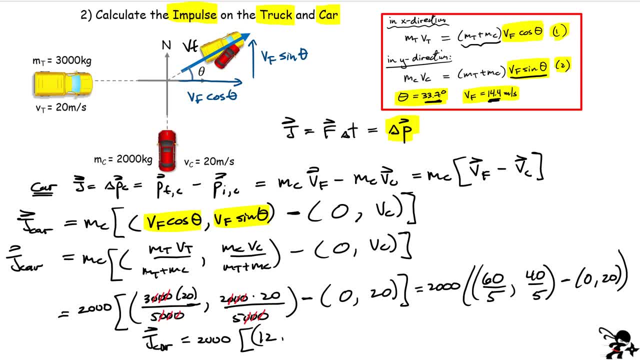 So that there is 12.. All right, That is that x component. And here what do you have? 40 over 5.. 40 over 5 is 8.. 8 minus 20 also gives me- Well, that's going to be negative- 12.. 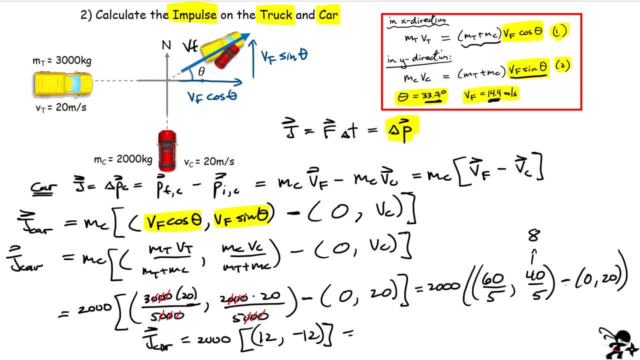 Okay, And I still have to multiply by the 2,000.. All right, So that's easy to do So. at the end, the total vector for the impulse on the car becomes 24,000 and minus 24,000. 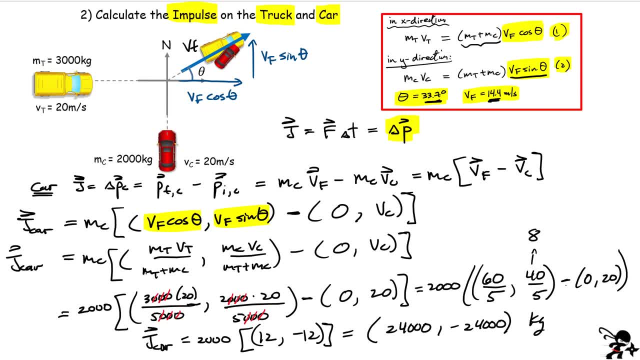 Okay, And again, that comes in units of change of momentum, which is kilograms, meters per second. That is the impulse on the car. Now does this make sense? This is a vector pointing in which direction? Think about it. This here, this vector here, if I was just going to plot it, it has an x component and it has a y component, which is negative. right, 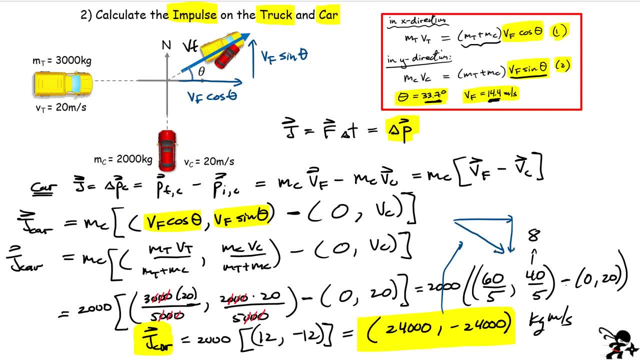 This is the direction of the impulse on the car. Okay, So this is J car. All right, Let's go ahead now and look at the impulse on the truck, All right? So the last problem now is we look at the impulse on the truck. 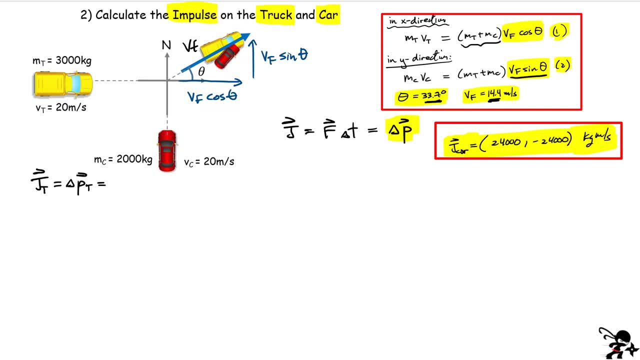 Again we have to look at the change of momentum, but only of the truck Mass of the truck, V final of the truck minus the initial momentum of the truck. So I just write it as Vt. So again, this is. 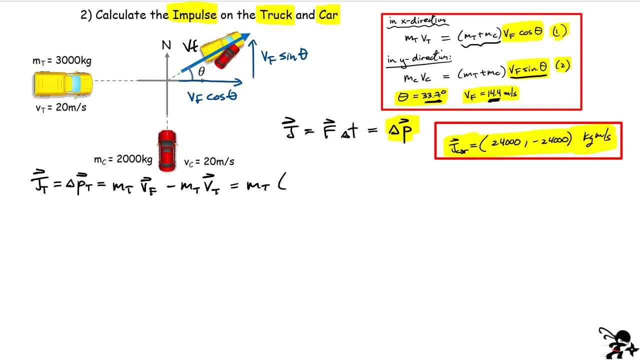 I have to write everything as a two-dimensional vector. We proceed the exact same way. Factor out the mass. We have this change of velocity here. So let's write down each of these as two-dimensional, Two-dimensional vectors: Our final velocity and our initial velocity. 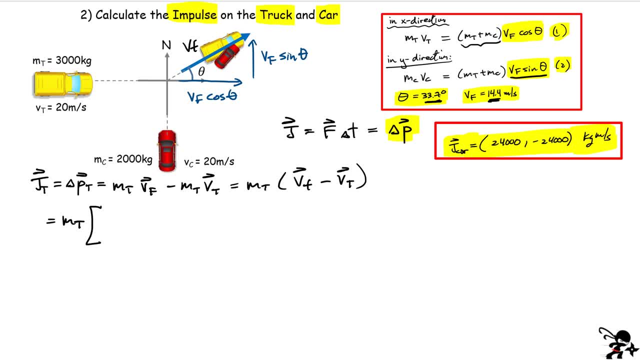 We have mass of the truck Square bracket. All right, What is the V final? That's the exact same as what I had for the car right. This is V final cos of the angle theta. V final sine of the angle theta. 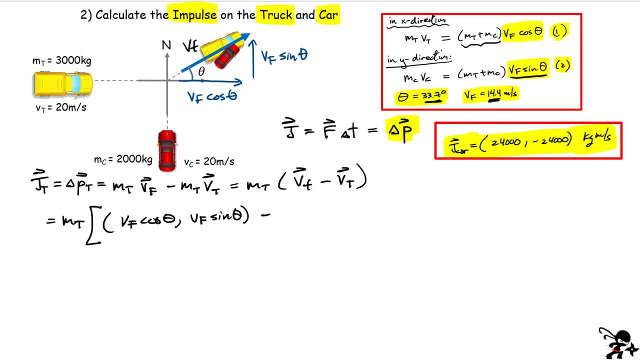 Minus, what is the initial velocity of the truck? It only has this east component, this x component, So I simply write this as Vt and zero. It has no north component. Okay, So let's take the difference between both of those. 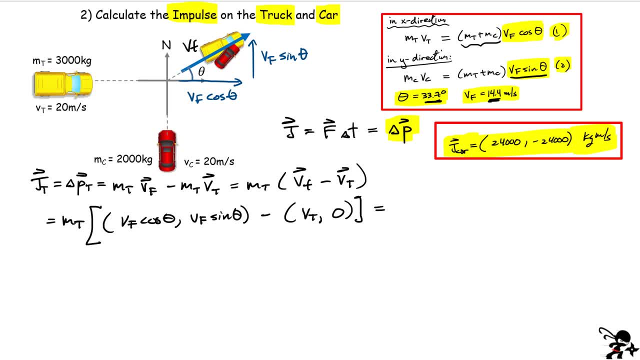 Now again, I'm going to do the substitution where I eliminate Vf cos and Vf sine, where I can write it only in terms of the masses. Again, you could substitute the numbers here. I just Sometimes, if you only keep three significant figures, you might find that the numbers might be a little bit different. 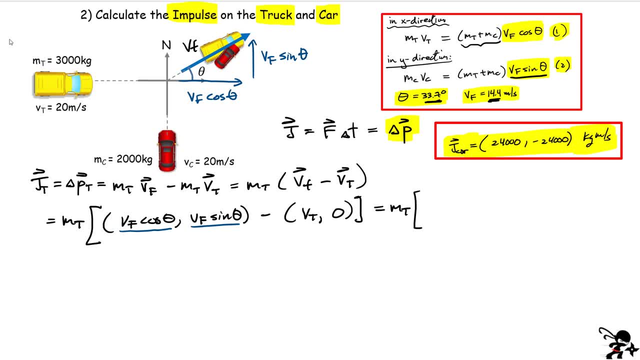 And I don't want to do that right now, So I am not going to do it. So Vf cos theta. Again, I can write that as minus. I can write that as mass of the truck. Initial speed of the truck. 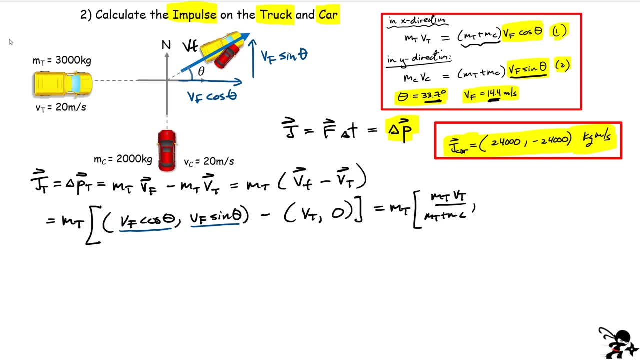 Divided by the total mass. Okay, The y component. You can write it as mass of the car, Speed of the car over the total mass Plus mass of the car. Alright, And minus this two-dimensional vector V of the truck is zero. 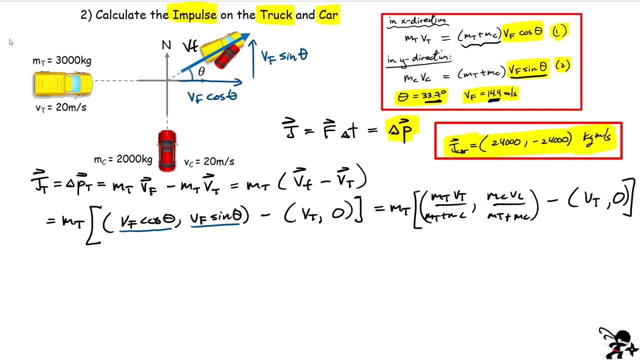 Alright, Now we can substitute our values, Because everything is known Right. There is no approximation here anymore. Mass of the truck was 3,000.. I open up this big vector Vf. So this is 3,000.. 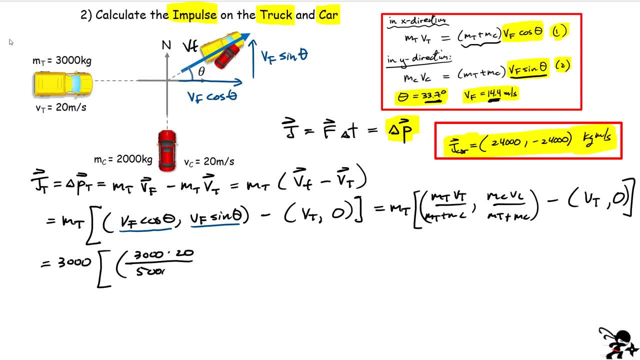 Times 20. Divided by 5,000.. The next one, 2,000.. Times 20. Over 5,000.. And minus that initial speed of the truck, Which is 20.. And it had zero component in the east direction. 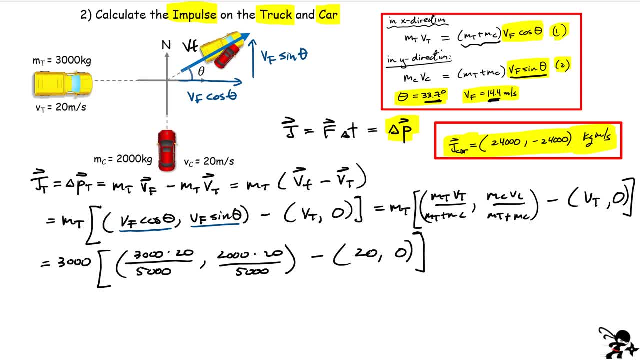 Again, Let's factor out a whole bunch of those zero terms. There is 3,000.. We can simplify that. All these three can simplify with those ones. Let's take the difference now between all of those terms. Keep the mass of the truck on the outside. 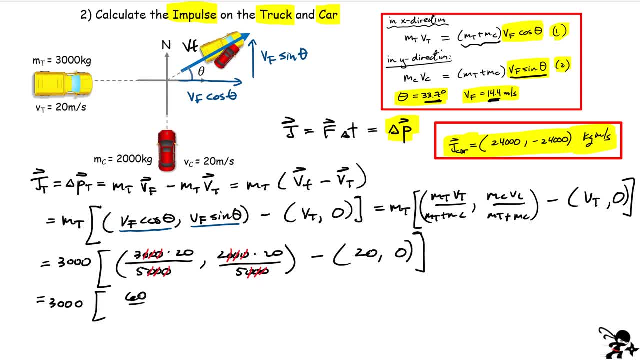 Alright. So what do you get? Three times 20 again gives me 60 over 5.. You can see these are some of the same numbers that we previously had. This is 40 over 5.. So that's that initial velocity. 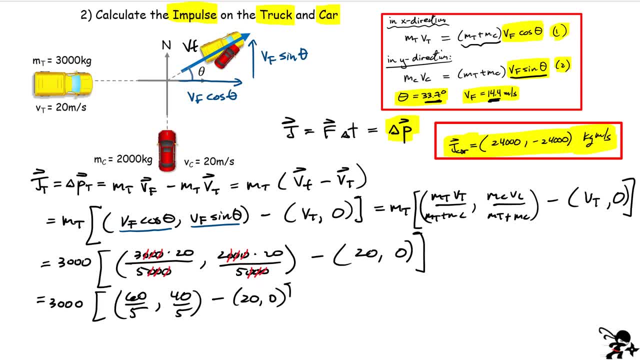 And minus 20 and zero. Okay, So we have 3,000.. Alright, Look at this. 60 over 5 is 12.. 12 minus 20.. 12 minus 20 again is going to be my minus 8.. 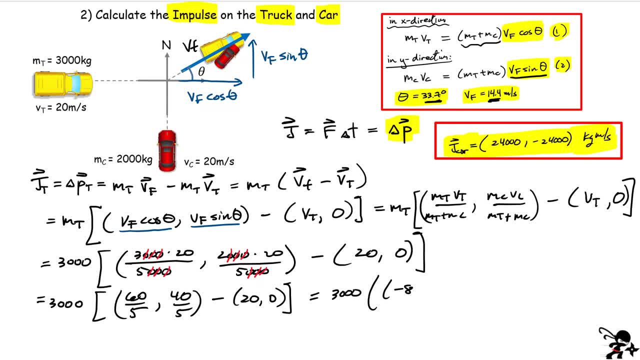 Okay, That's our x component for this vector And the last one. Actually, let me just clean this up here a little bit. This is minus 8 for the x component, And the y component now is 40 over 8 minus 0.. 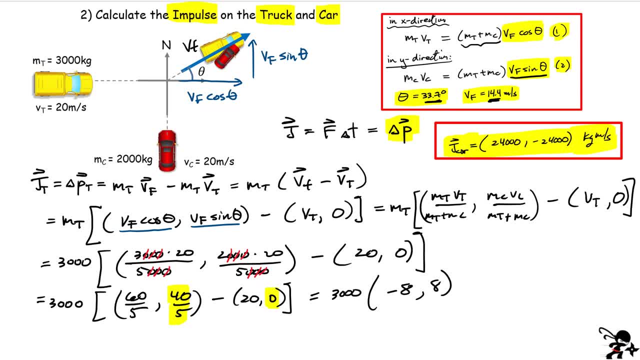 Okay, 40 over 8 is 8.. So you multiply through now by the mass of the truck And look what we get. We get minus 24,000.. And plus 24,000.. This is Write down, my final expression. 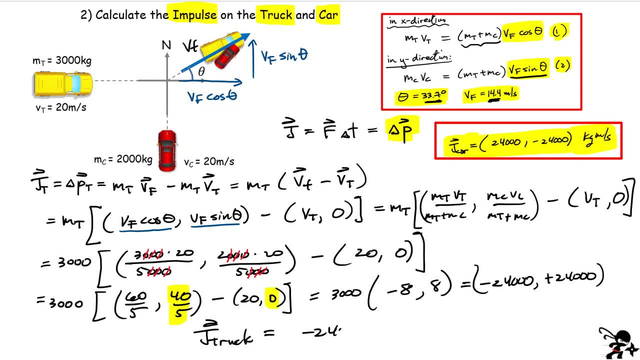 The impulse on the truck Is minus 24,000. And positive 24,000.. Those are the two components of the vector. Again, If you were going to now consider that, Compare it to the car. Look what we get. 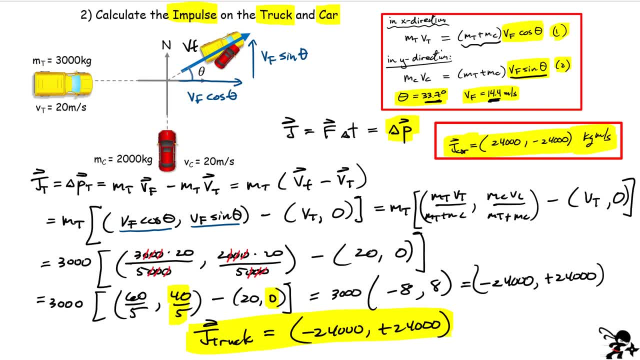 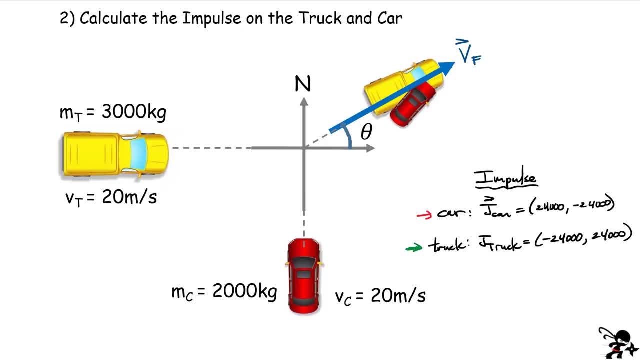 Alright, All of the components are the same, But it's in different directions. Let me go on the last page and just plot everything out So we can see what the vectors look like. Alright, So let's kind of look at everything, just as the vectors.